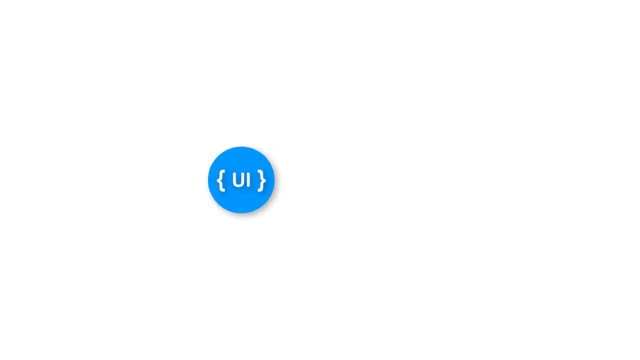 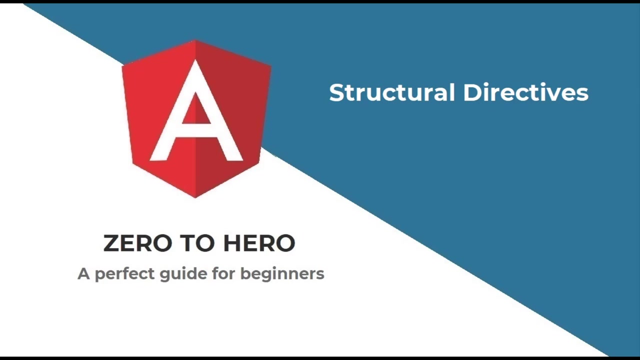 Hi friends, welcome back to the brand new series on Angular zero to hero: a perfect Angular guide for beginners. In my last video, I have explained about data binding in Angular. In this video, I'm going to explain about directives. Directives in Angular can be. 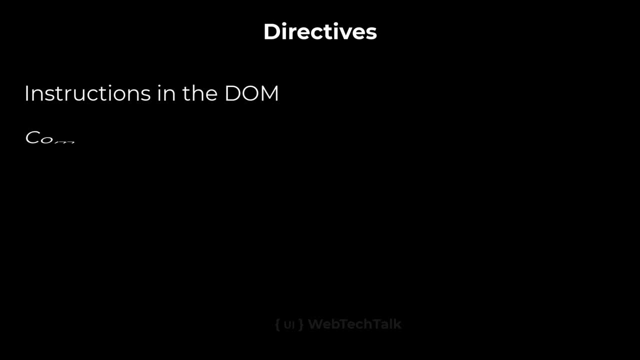 defined as instructions in the DOM. Angular components are also directives because through component we are instructing Angular to place the HTML and TypeScript logic in the place of the selector. So components are also directives, but with a template. Apart from component, we have two types of inbuilt directives in Angular Structural directives attribute. 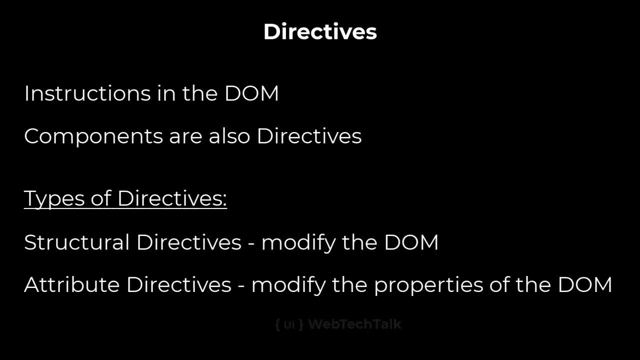 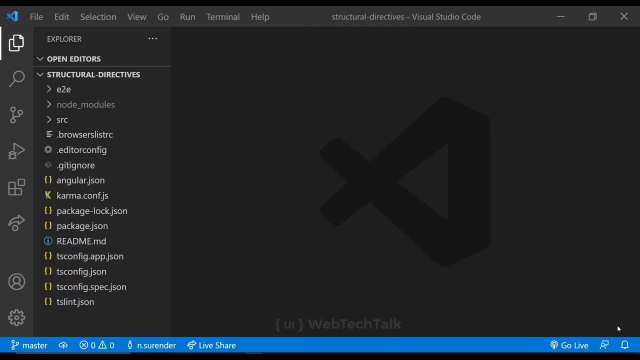 structures, Structural directives or directives, those modify the DOM. Some of the most common structural directives are ng-if, ng-for and ng-switch. Let me explain in detail using an example program. I have created a new Angular program using CLI. I have also started the 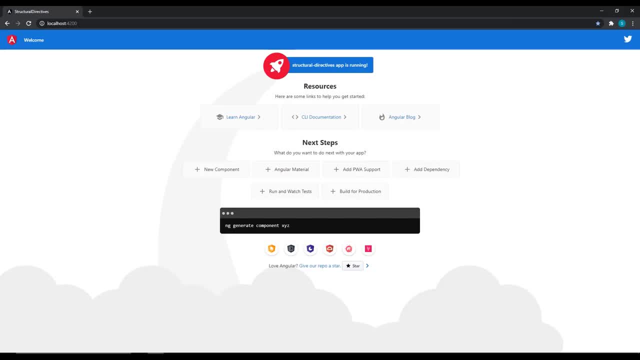 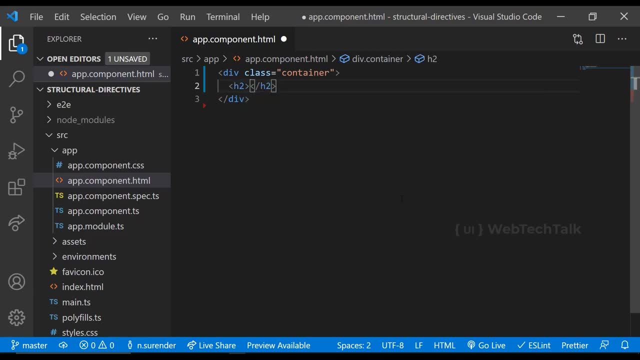 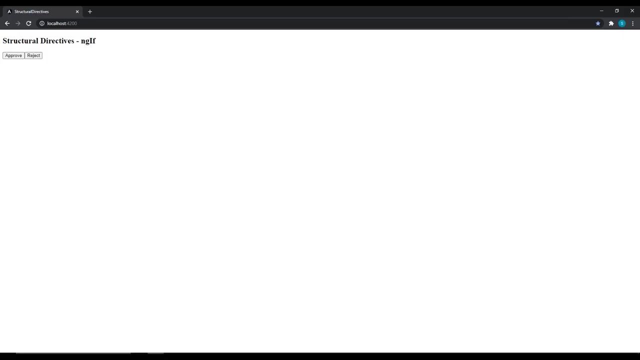 server and opened the application in a browser. Now I'm deleting the existing code in app component HTML. I'm adding a container div and then a heading, followed by row and column divs. Inside that, I'm creating two buttons: approve and reject. We can see this If we add bootstrap to our 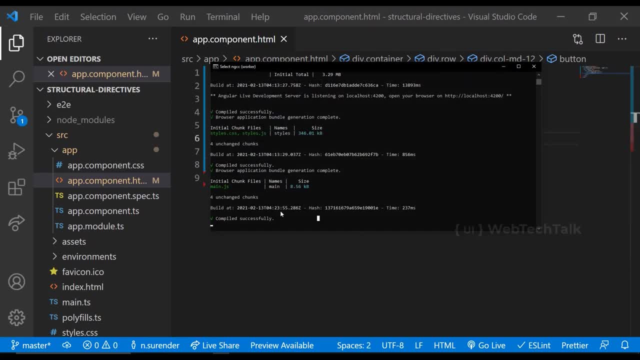 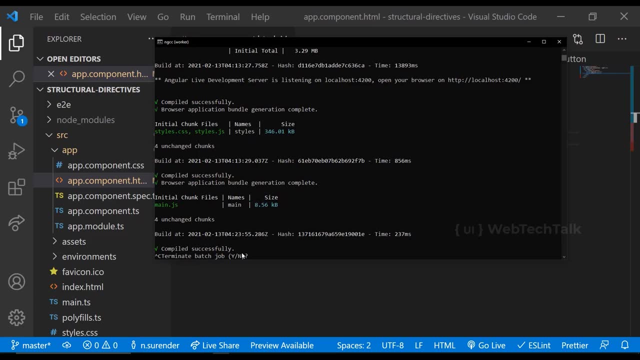 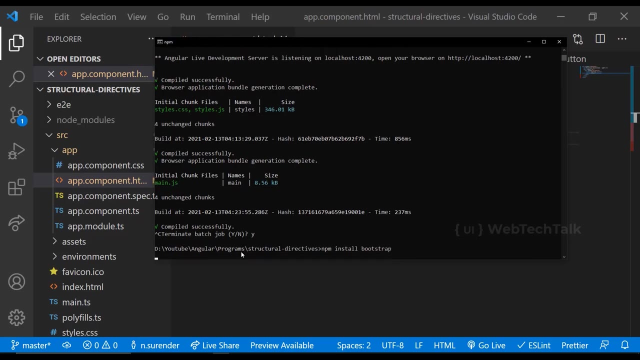 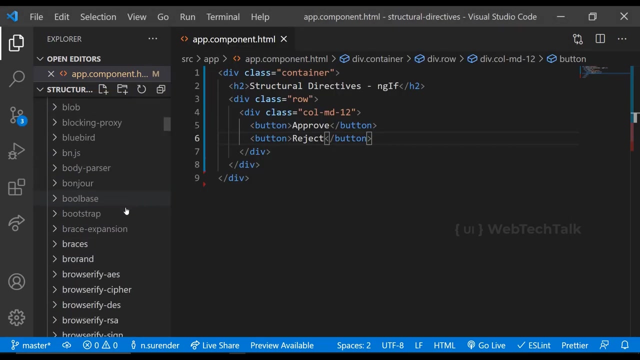 application. we can apply styles easily. So let's see how we can add bootstrap. I'm opening the command prompt, stopping the server using control C and then installing bootstrap using npm. npm install bootstrap. Now bootstrap has been installed. We should see this in node modules folder. We have the. 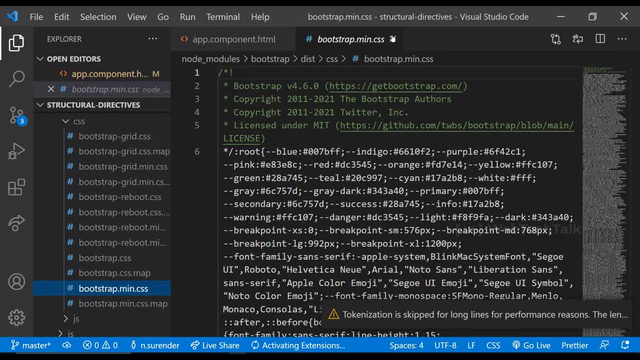 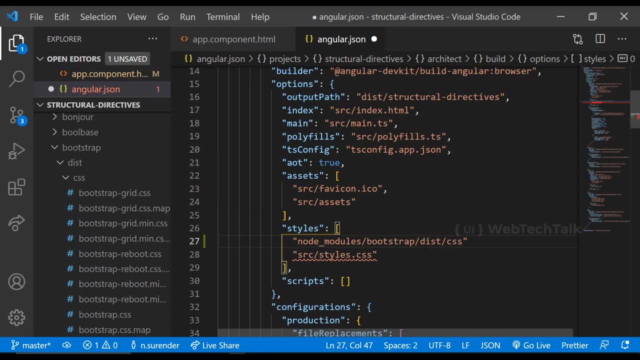 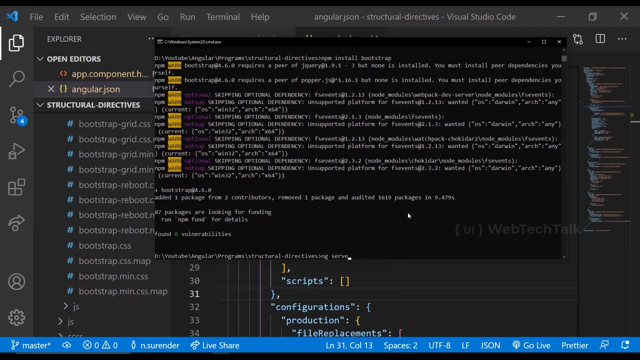 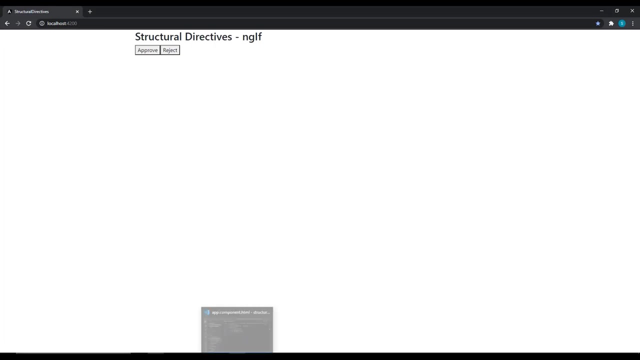 bootstrap CSS here. We need to add this path to angularjson. That's it: Bootstrap has been added and now we can start the server again. if i refresh, we can see the bootstrap styles for container, row and column classes have been applied. now let me add some styles for buttons. 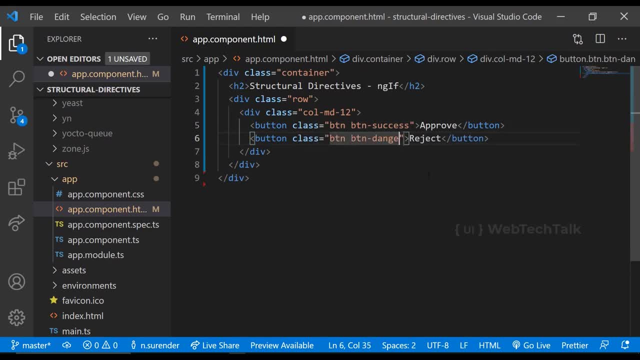 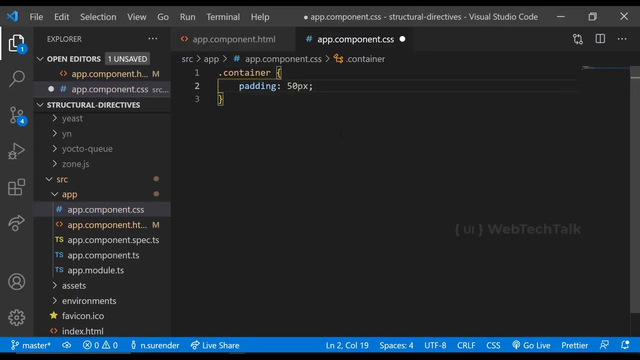 using bootstrap classes and then in app component css, i'm adding some styles: padding: 50 pixel text align center and a height of 2000 pixel to the container class and a margin of 40 pixel to the h2 class. the width of 130 pixel and margin 20 pixel to the. 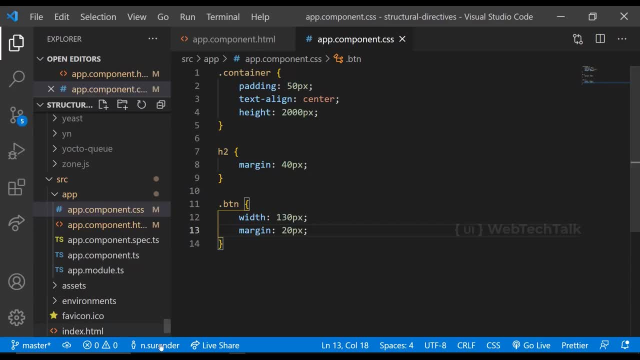 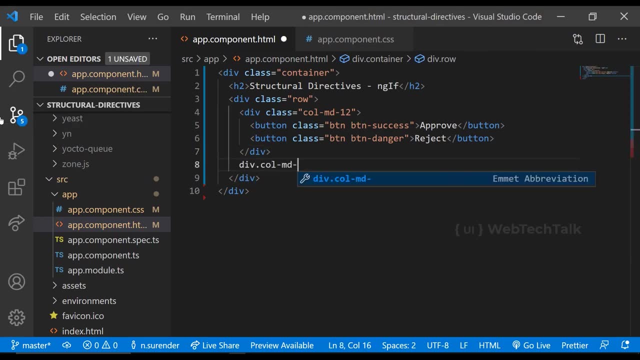 button class. let's preview once now. i wanted to show different messages on clicking these buttons, so i'm creating another column view inside that i'm creating two paragraph tags. in the first tag i'm having the tag. in the first tag i'm having the tag text: your application has been approved and. 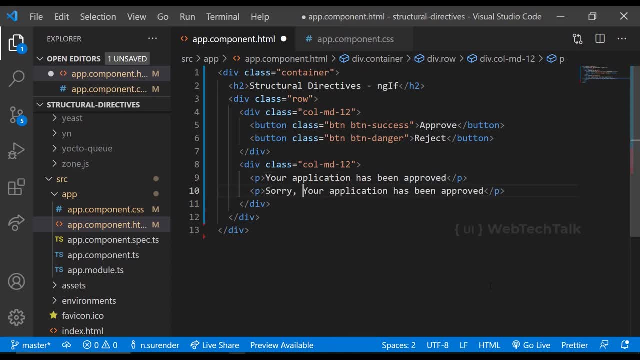 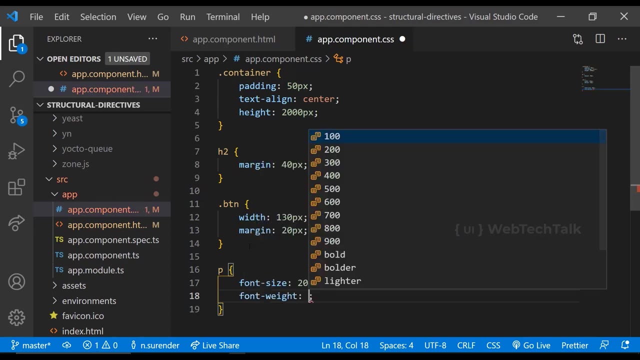 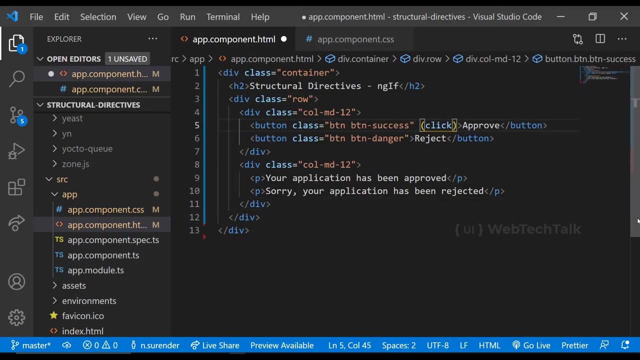 in the second paragraph i'm having the text. sorry, your application has been rejected. in preview we can see both the text. let me also increase the font size. okay, now i want to show the message based on the button click. for that i am adding click even to the buttons. 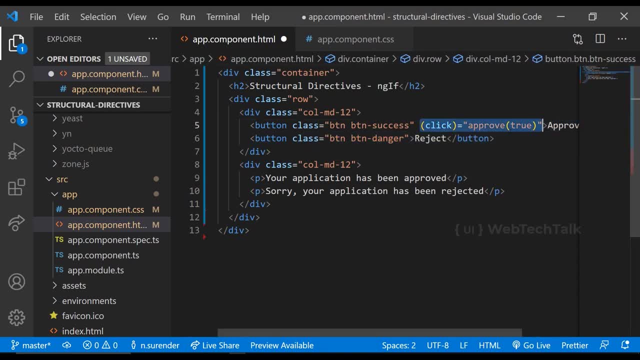 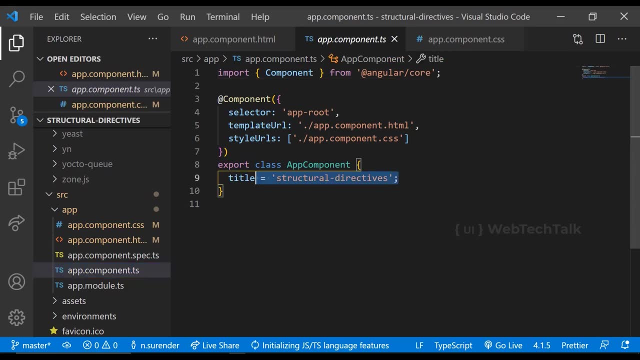 and calling a function: approve. for the approve button, I'm passing the value as true and for the reject button, I'm passing the value as false. and in the typescript component, let me create the approve function and I'm also creating a boolean variable is approved and defaulting it to false. 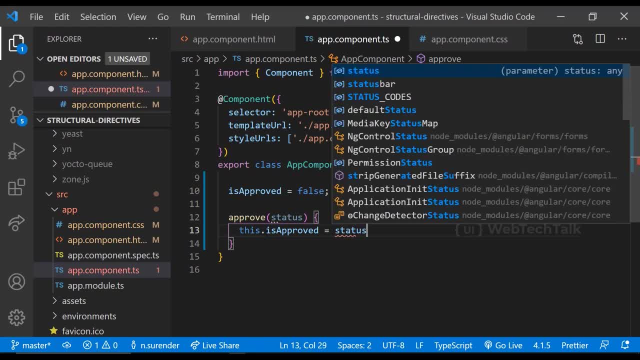 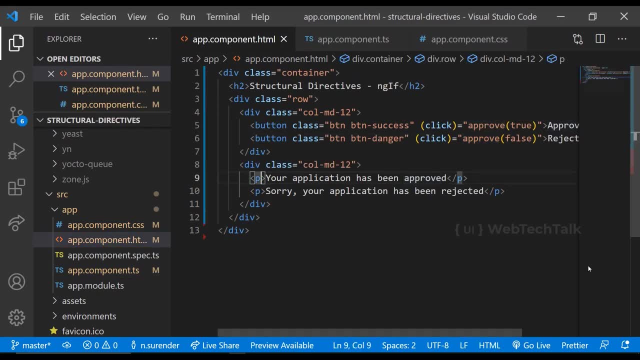 inside the approve function, I'm getting the value from html component and assigning to this variable. coming back to the html, I'm adding a structural directive, ngif. please note here the syntax of any structural directive will be starting with a star. this is mandatory and this is to inform angular that this directive is going to modify the DOM. 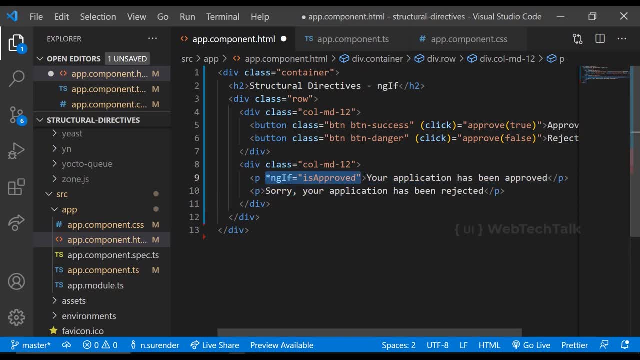 and ngif accepts any variable or expression which gets transformed to a boolean. so for the first paragraph I'm adding is approved and I'm adding a boolean. and for the second paragraph I'm having a not or negation operator followed by is approved. now we can see only one p tag is visible now. 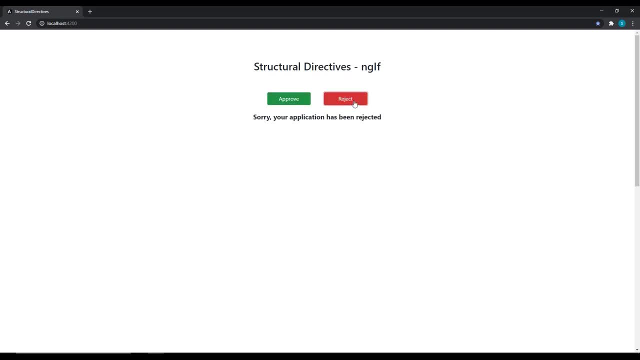 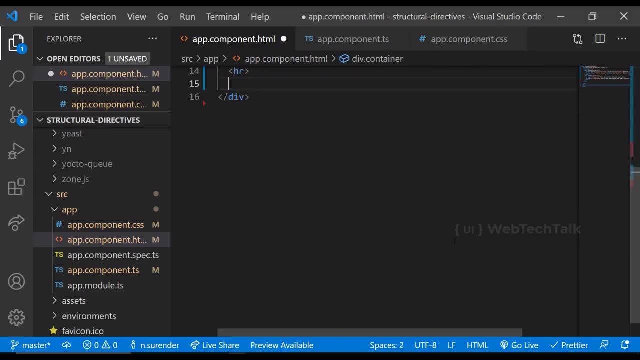 and on clicking the other button, the other message is visible. this is how we can use ngif to hide and show any DOM elements dynamically. now let's move to ng. for using ng, for, we can loop through an array and display that in the html. for that, I'm creating an array called numbers. 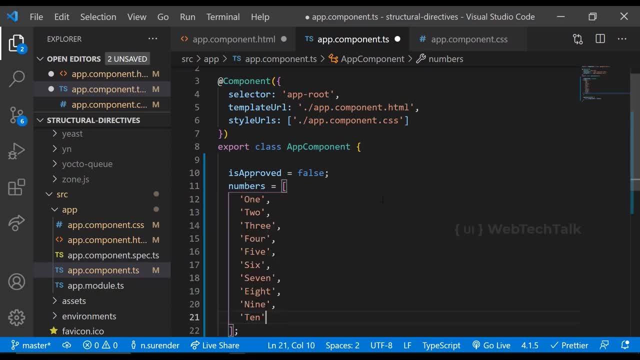 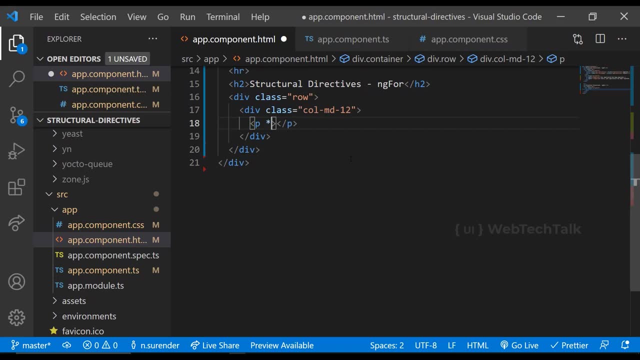 in numbers array. I'm having the numbers from 1 to 10 now in html. we can display these numbers one by one inside p tags. for that we can use ng for. ng for is also a structural directive, and so we should not forget to add star. 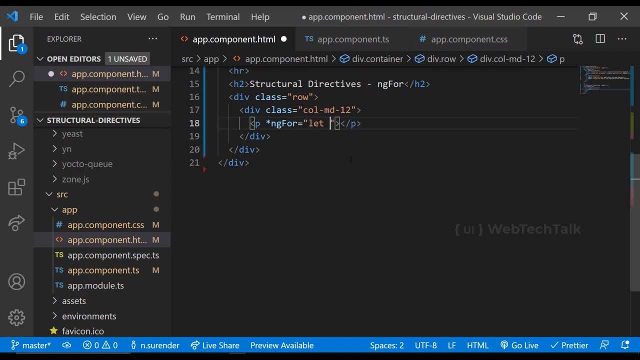 in ng, for we can loop through the array like let number of numbers. here numbers is the array we have declared in the typescript component and number is the variable which we can use to add numbers to the array. we can use it in html and inside p tag. using string interpolation we can display the number. 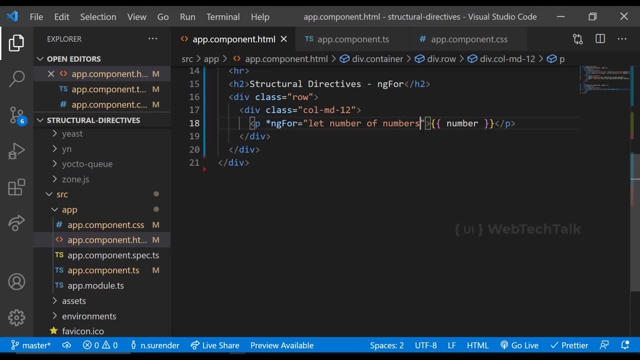 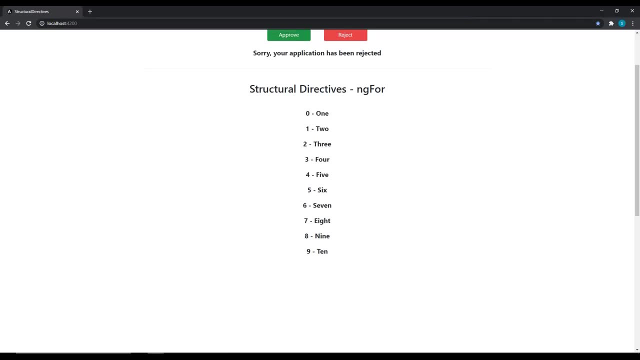 we can see. all the numbers are listed one by one in ng for we can also access an index and use it if needed. index always starts from zero, so if we need to start this from one, we can increment it before displaying. this is how we can use ng for to loop through an array and display. 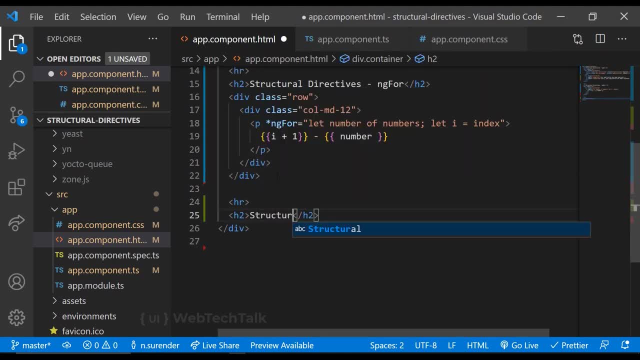 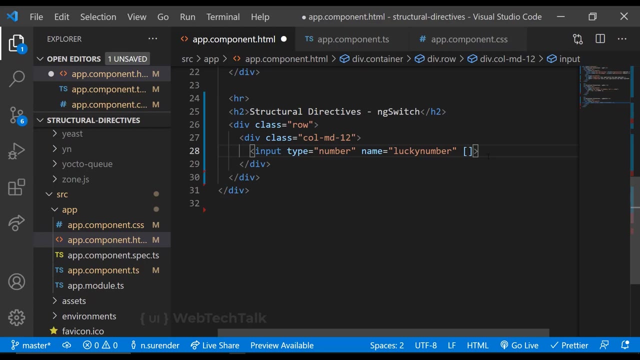 them in the html. next, let's move to ng switch. using ng switch, we can switch between different dumps based on some value. to explain this, let me create an input element which accepts only number and I'm binding this to a variable called lucky number using ng model directive. 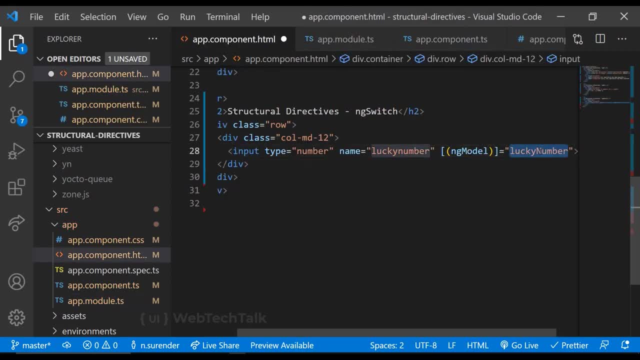 remember we need to import the forms module, otherwise this will not work. and in the typescript component I'm creating that variable and assigning it to zero. back in html, I'm creating a column div in which I'm using the ng switch property and binding that to the lucky number variable using property binding. 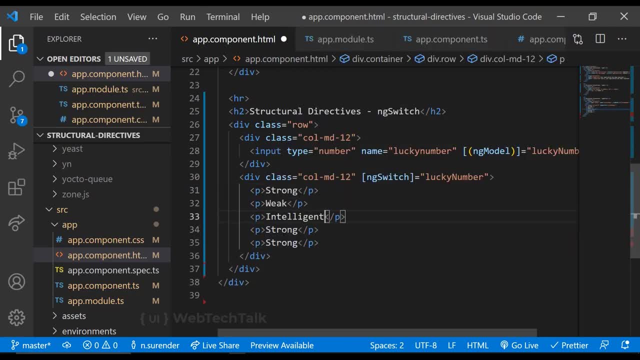 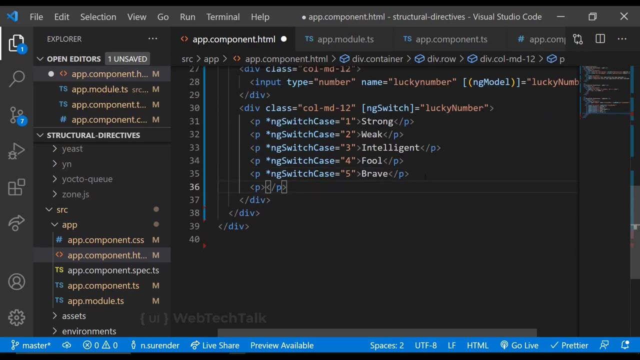 inside that, let me create p tags to display words. I can switch one of these words using ng switch case. for the case statement, we need to add star, also assigning the values from 1 to 5, and then we can also default something using ng switch case.